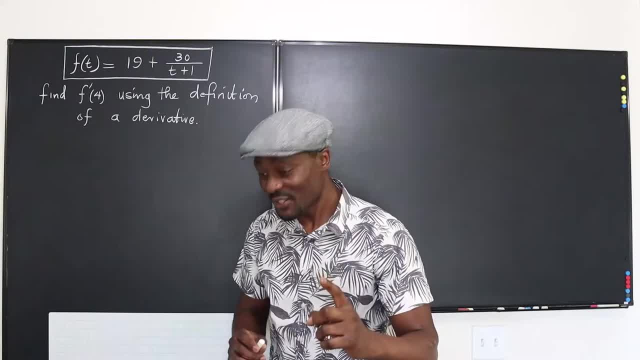 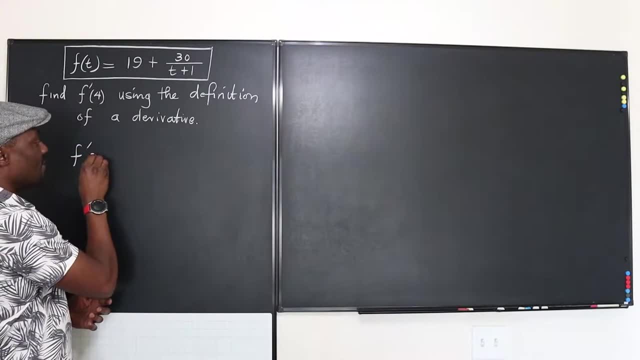 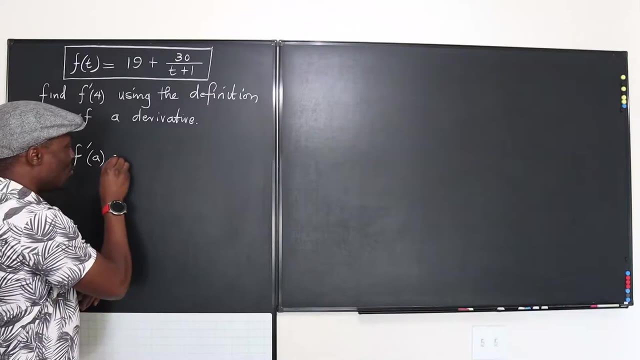 is basically the limit, So let's just write it. We know that the derivative of this function at a point a- because there has to be a point where we're taking the derivative, Let's say that point is point a- is usually defined as the limit. 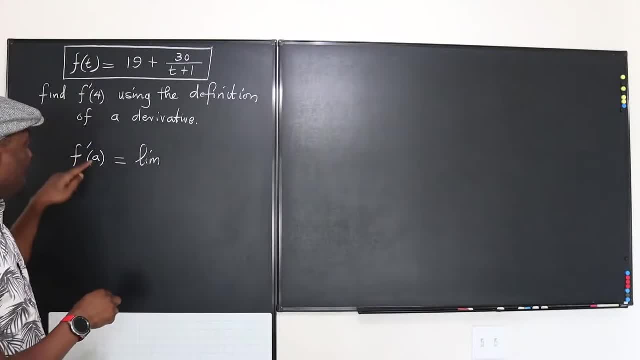 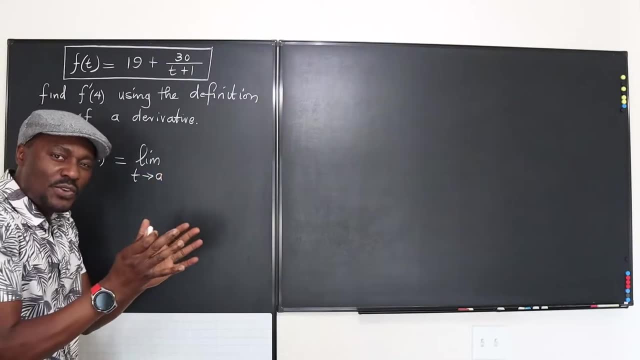 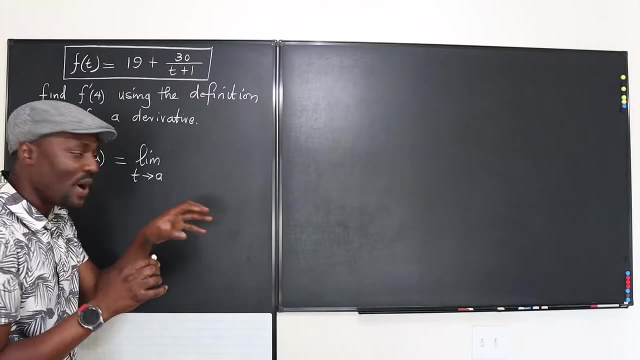 Okay, as your independent variable is approaching that point. as your independent variable approaches that point, the closer you get to that point, the more accurate your answer will be. So that's the idea. What number would you get? Well, it would be basically the function minus the value of the. 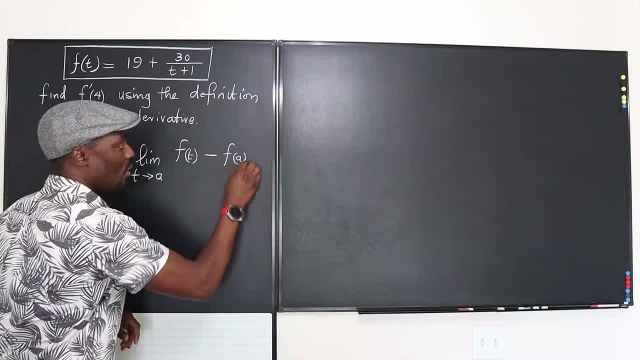 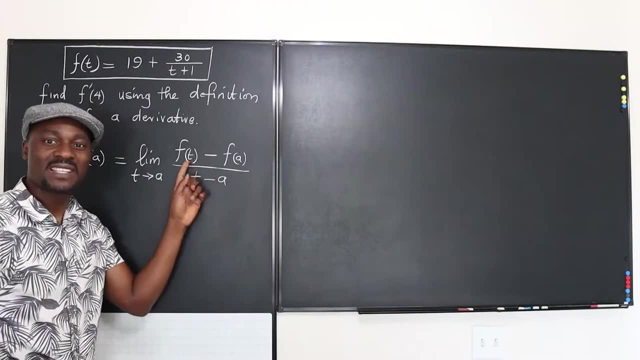 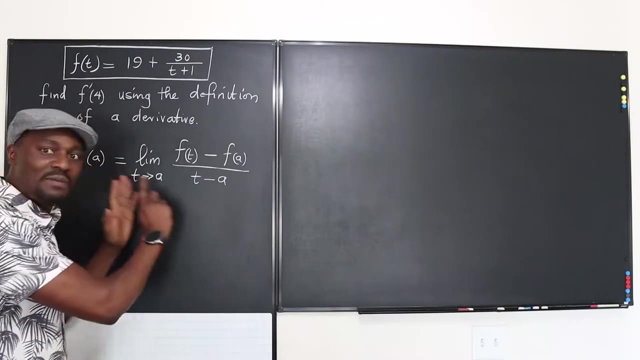 function when you get to that point, which is f of a divided by the difference, the distance between your t and that point, a. So remember, sometimes this is x, it's any variable. usually we do t or we do x. Okay, but just know, this is the definition. All you have to do after knowing this is just do your. 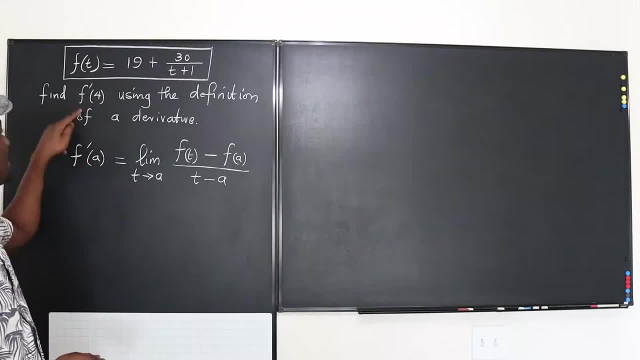 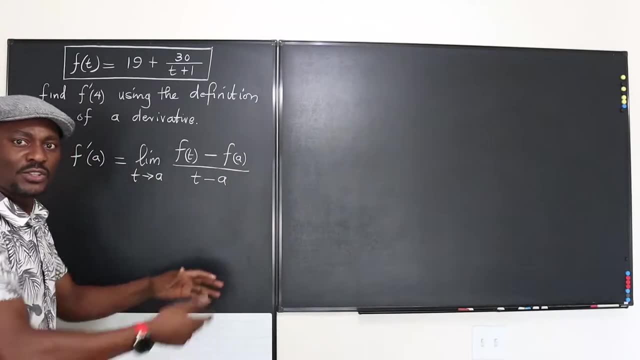 substitution. Now we know that a is 4 in this case, because we're supposed to take the derivative at the point, t equals 4.. So let's put the numbers in here and just do the algebra. That's all. So at this point, f, prime of f is: 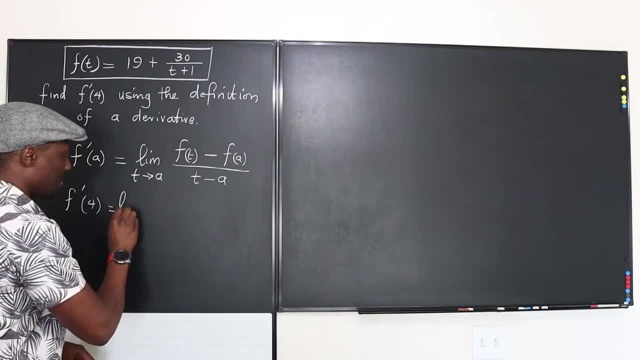 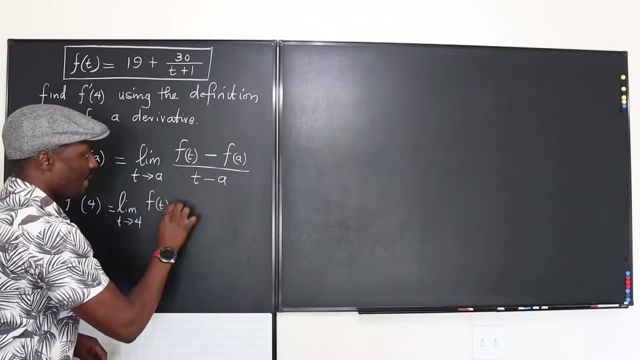 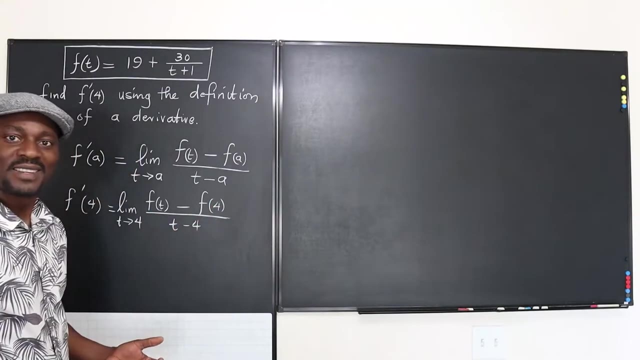 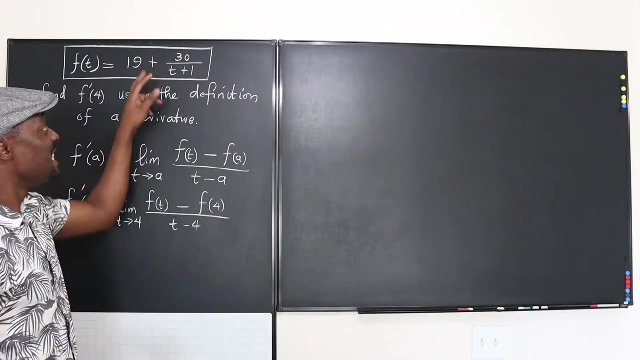 4 is going to be the limit as t approaches 4 of f, of t minus f, of 4, divided by t minus 4.. Beautiful. So what is f of t? Well, that's it. And what is f of 4?? It is still this, It's just. 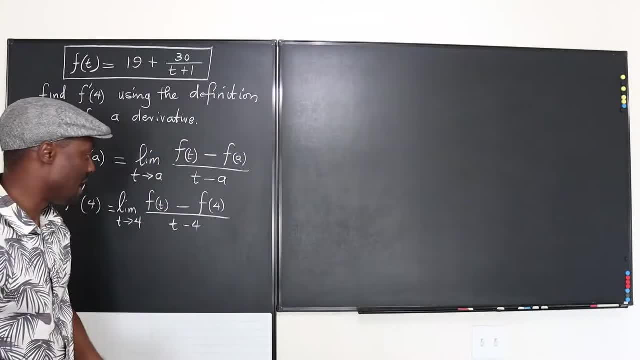 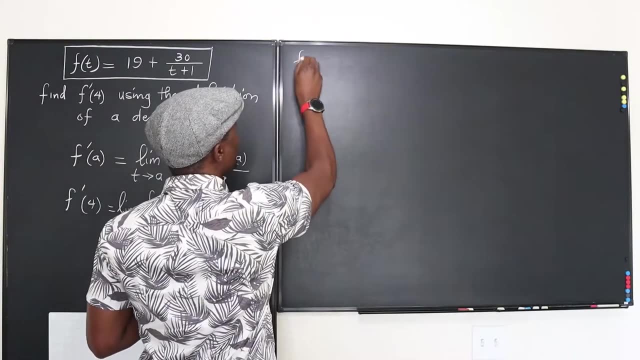 that, instead of writing t, you're just going to put 4 there and simplify and that's it. Okay, now let's go. So this is going to be the same thing as f. prime of 4 is going to be the limit. 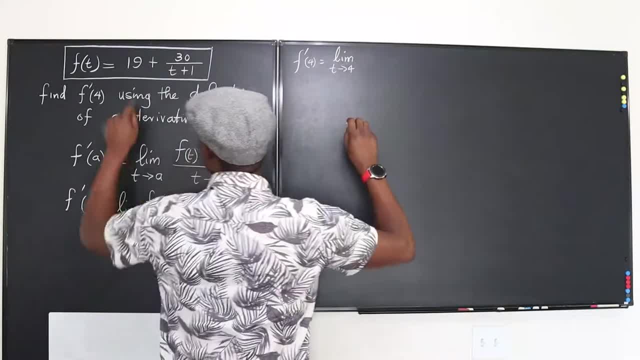 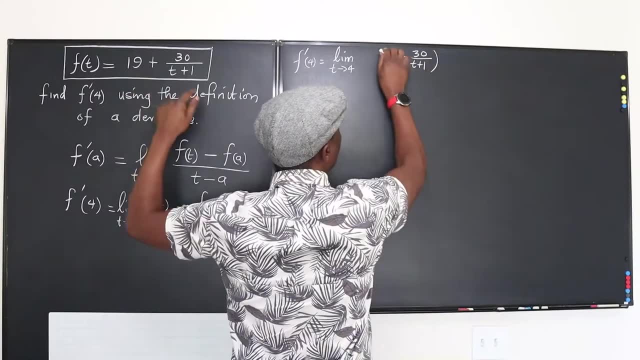 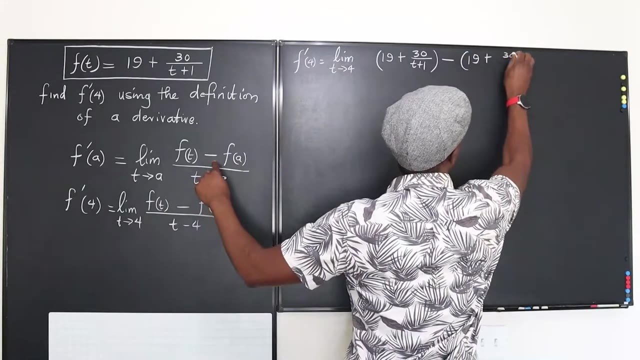 as t approaches 4 of the function itself, which would be 19 plus 30 over t plus 1, okay, minus, this is going to be 19 plus plus 30 over. we're not going to use t this time, we're going to use a. that's going to be. 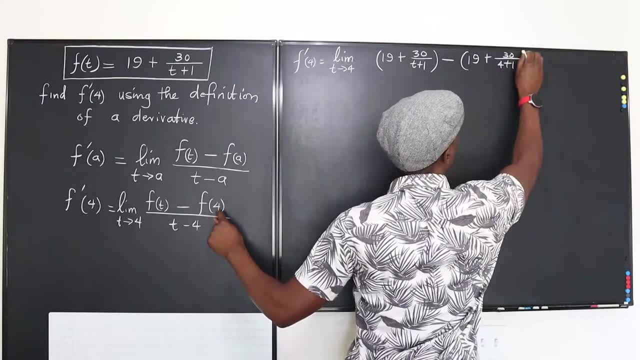 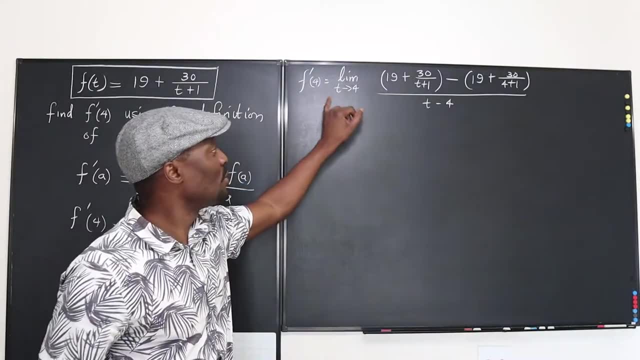 but what is a is 4,, that's 4 plus 1, and then we divide everything by t minus 4.. So if we take the time to distribute what we have here, this is what we're going to end up with. 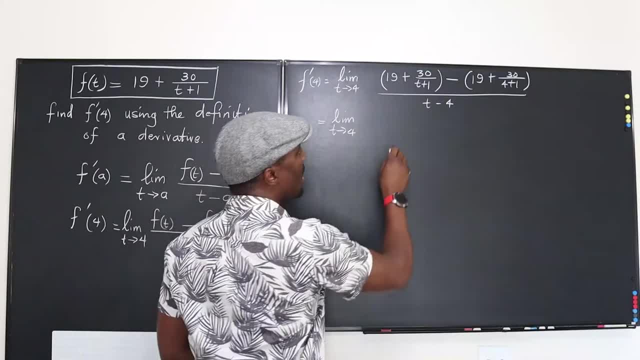 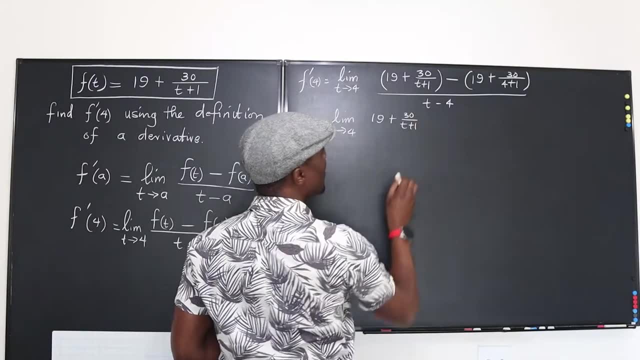 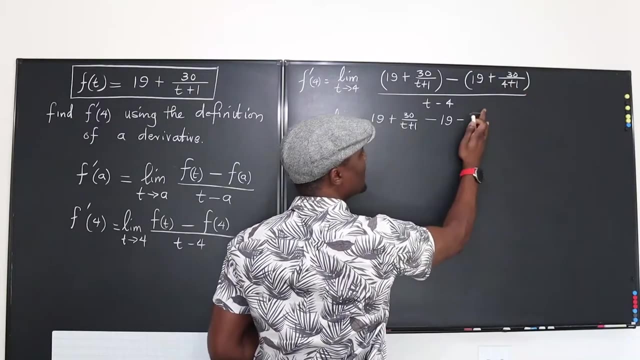 the limit as t approaches 4 of this is going to be 19 plus 30 over t plus 1, minus 19 minus 30 over, oh, 30 over 5 is just going to be 6.. Okay, so we're going to just write. 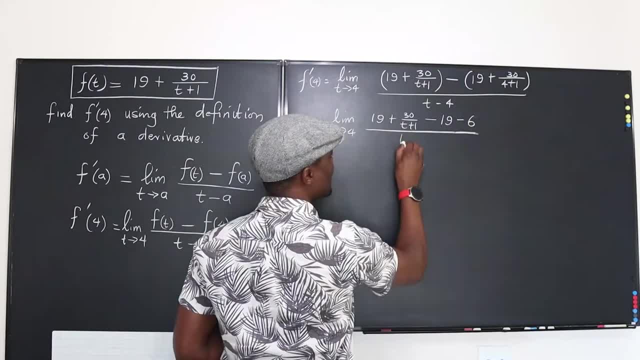 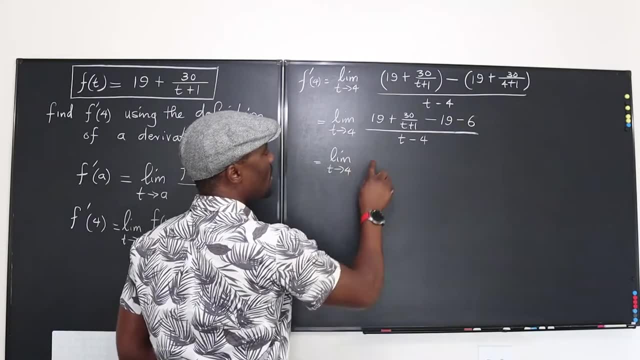 6, and we'll divide all of that by t minus 4.. Well, the next line is going to be the limit, as t goes to 4.. When you take care of what's on top here, what you're going to notice is that 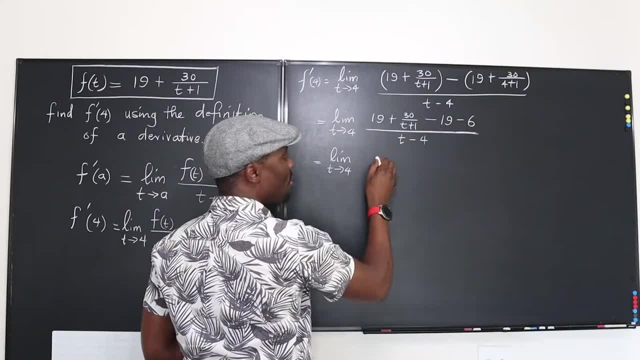 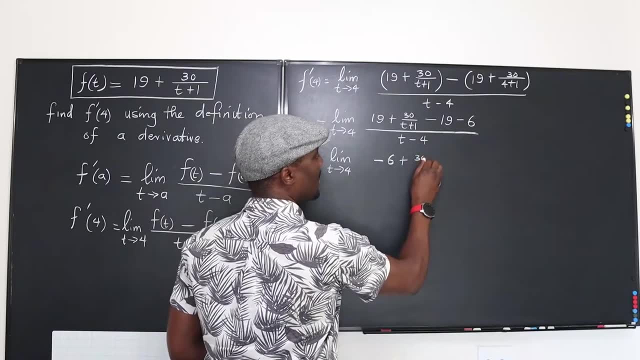 19 takes away 19, and you have this. so you're going to have- I'm going to put the negative number in front, so you're going to have. I'm going to put the negative number in front, so you're going to have negative 6, okay, plus 30 over t plus 1 divided by t minus 4.. 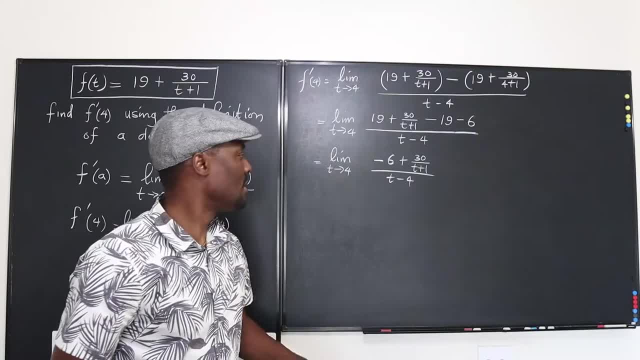 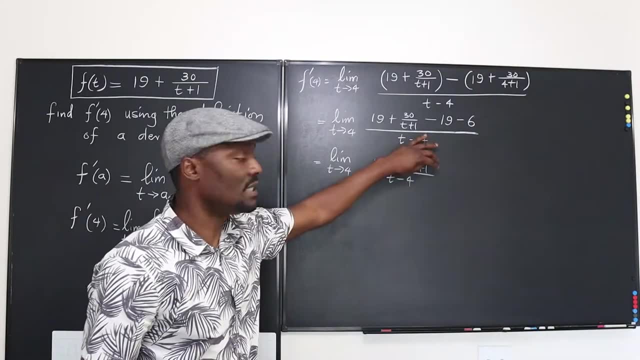 You will start saying: can't we just plug in this number, the 4 here? now? No, because if you plug in, t equals 4. right now what's going to happen is you'll get a 0 on top and 0 under. That means 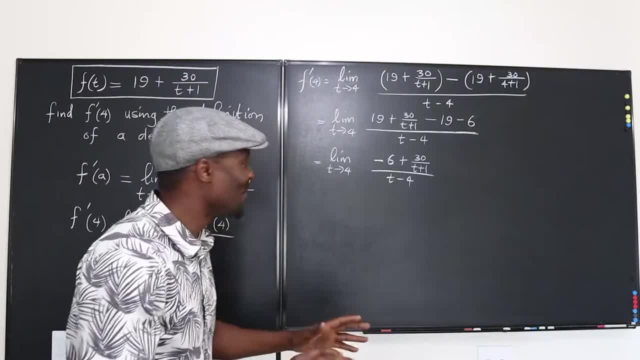 you still have some algebraic manipulations to do, so let's not do that yet, So let's go to the next stage. Now, what's the next stage? So let's go to the next stage. So let's go to the next stage. 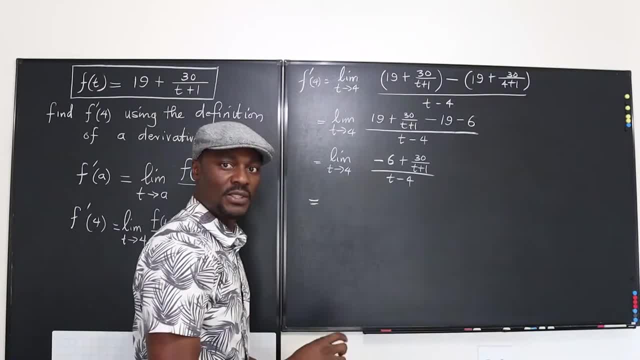 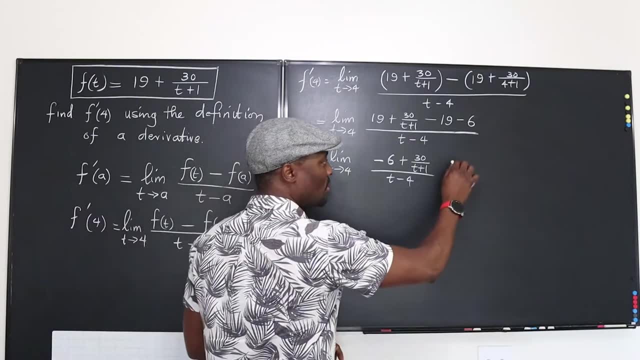 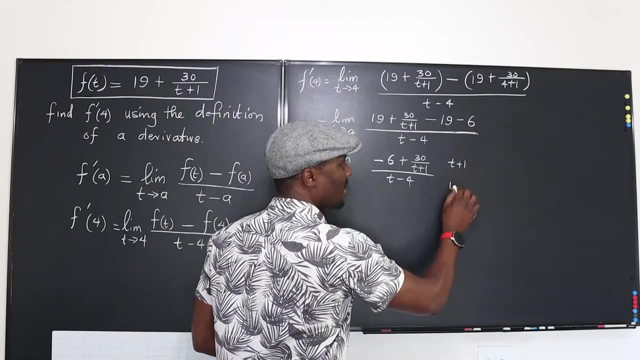 We're going to try and get rid of this fraction on top, this denominator on top. We want to bring it down, but this guy is standing alone. okay, So remember, the best thing to do is to multiply the top by what you're trying to get rid of in the top, which is t plus 1, okay, Also multiply this. 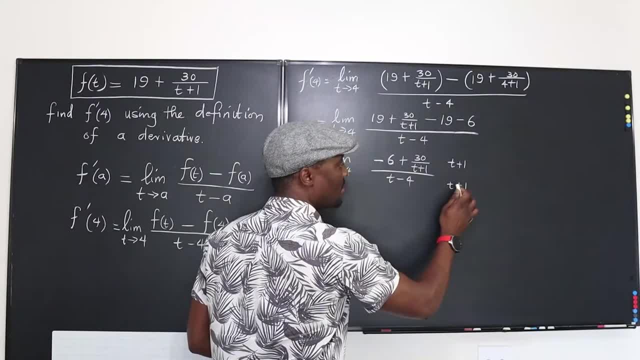 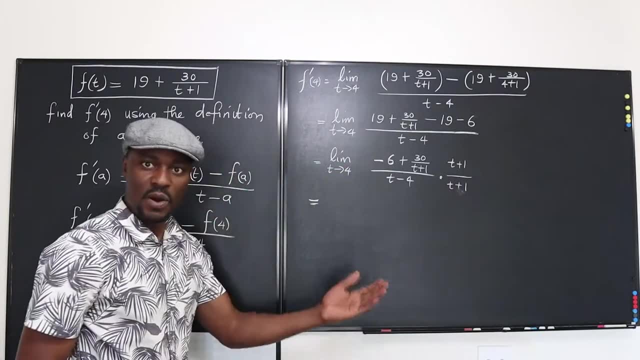 by t plus 1.. So you want to multiply both top and bottom by t plus 1,, t plus 1.. So you didn't change anything, You're multiplying. okay, That's still 1.. So let's multiply this by t plus 1,. 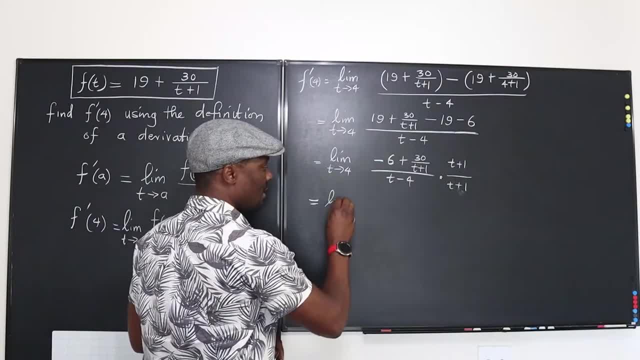 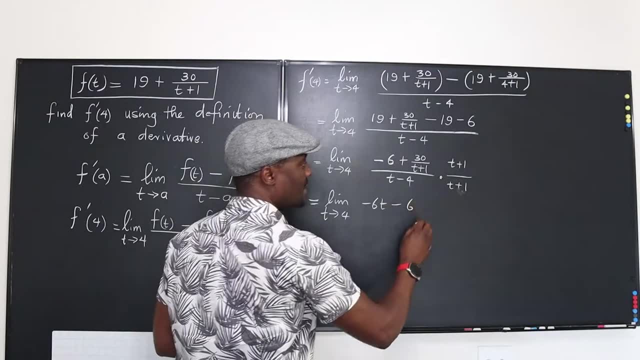 and by multiplying negative 6 by this, you're going to end up with the limit, as t approaches 4, of negative 6t. Negative 6 times 1 is negative 6, and 30,. well, this is now going to cancel. 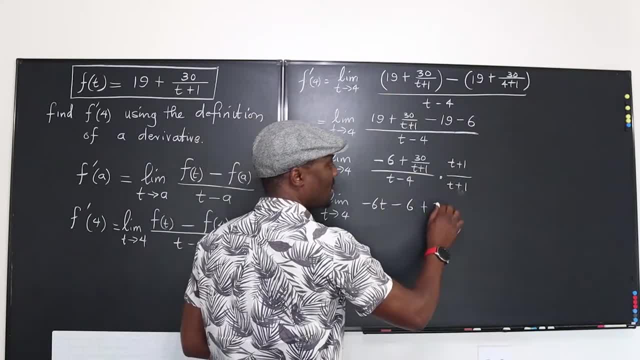 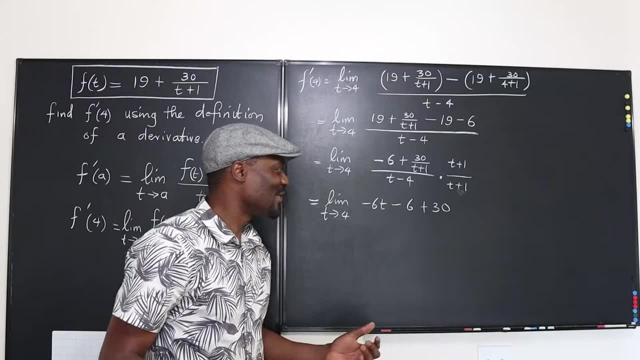 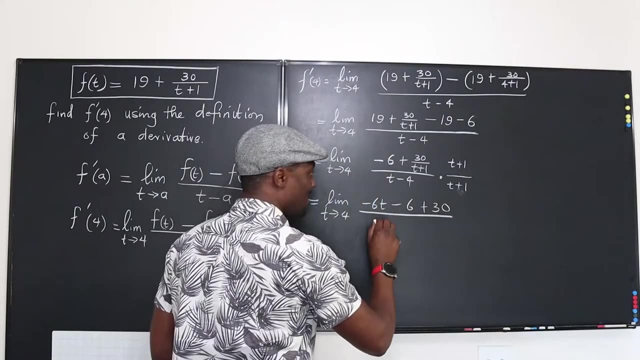 this out. This is going to take this out and you're going to have plus 30,. okay, Ignore the background noise you just heard. The AC just came on. I forgot to turn it off. Okay, Now divide it by: this is going to be t minus 4, and this is going to be t plus 1,. okay, So remember. 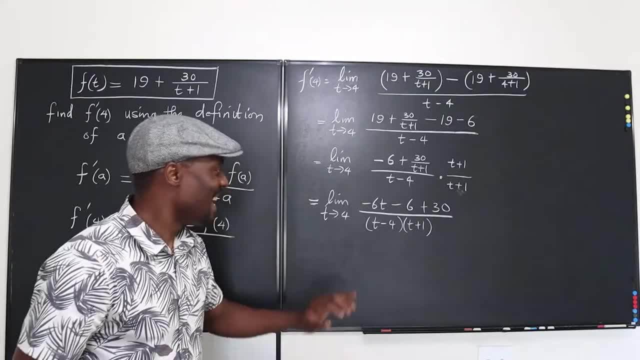 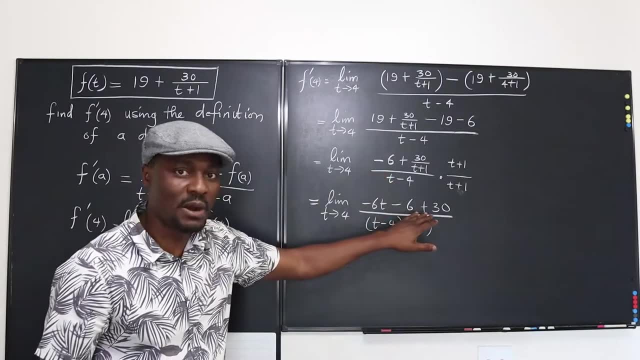 I told you there's still some algebraic manipulations to do. Yes, because we need to get rid of this thing giving us a 0 in the denominator and it's going to come from the top. Now look at what you have in the top right now. What you have is negative 6t minus. that's negative 6t plus 24.. 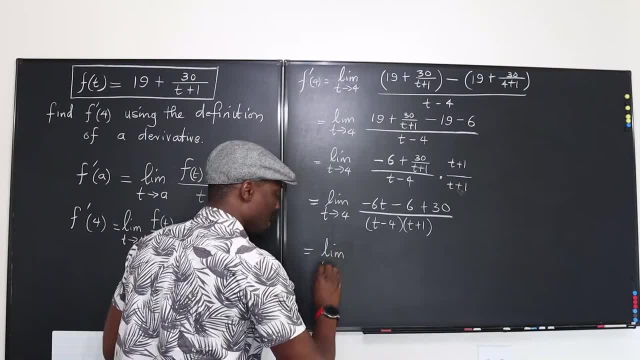 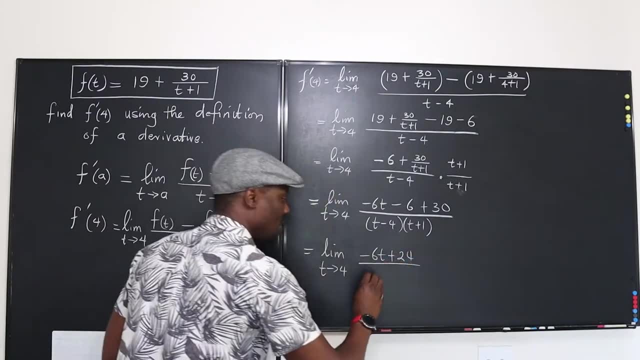 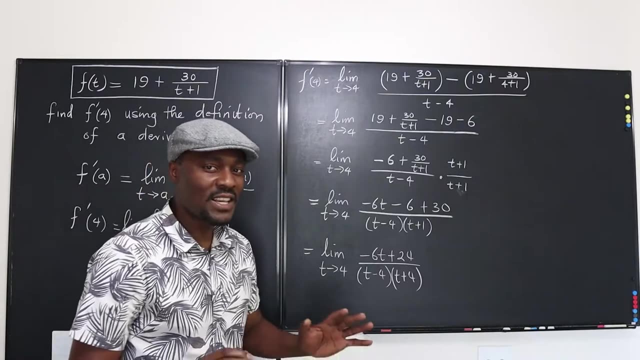 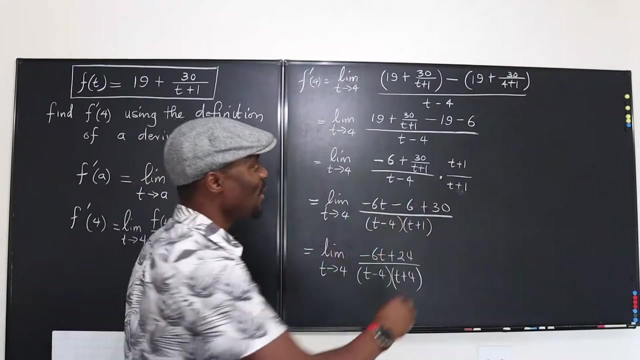 So we can rewrite this as the limit, as t approaches 4, of negative 6t plus 24,. okay, Over t minus 4, and this is going to be t plus 4.. So now I can clearly see that if I take out negative 6, it's going to give me t minus 4.. You see that? So I'm going to go over here. 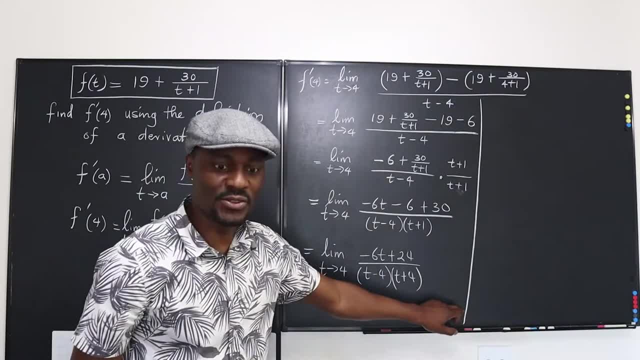 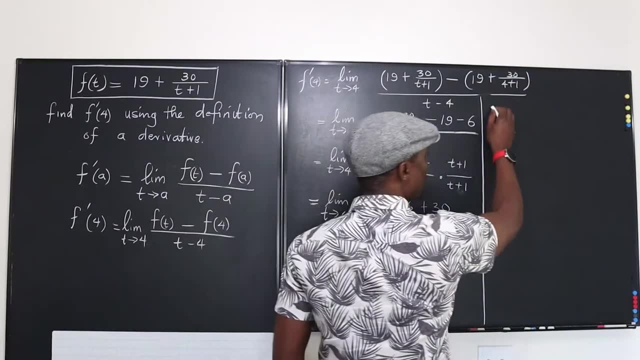 and I'll just finish the work. This is not a straight line. I'm going to fix that. I fixed it. So if we go over here, what we're going to see is that if we take out negative 6, we're going to 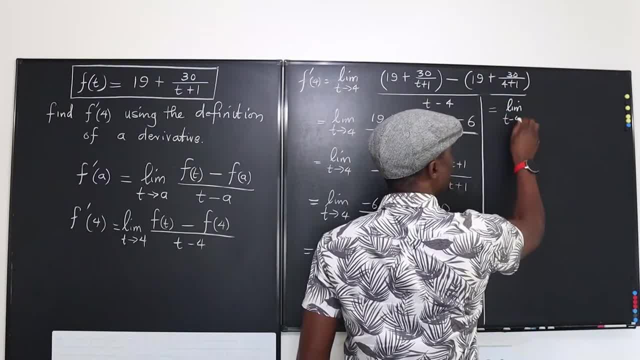 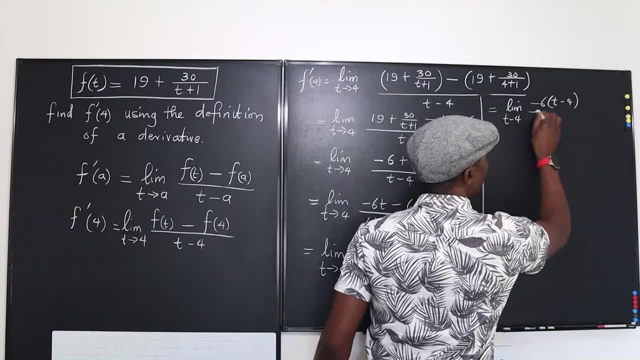 get the same thing as the program. This is the same thing as the limit, as t goes to 4, of take out negative 6, that's going to be negative 6 into t minus 4, over t minus 4, t plus no, t plus 1.. 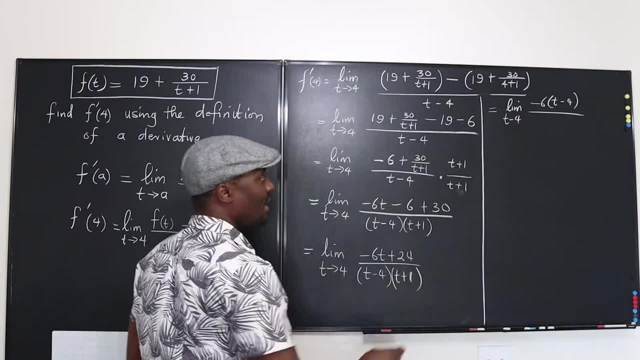 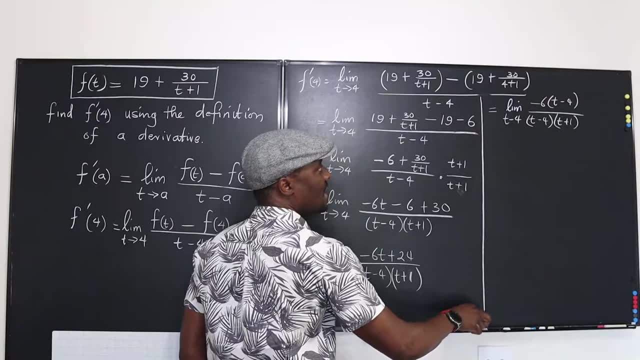 Sorry, This is t plus 1.. This is t plus 1, okay, So that's going to be t minus 4, t plus 1.. Okay, Obviously, this will take this out like that, and what you have to do is you have to. 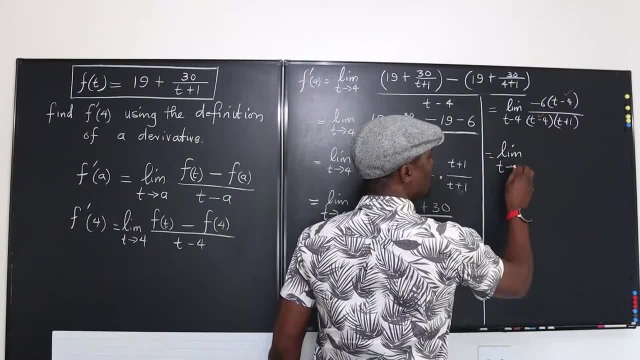 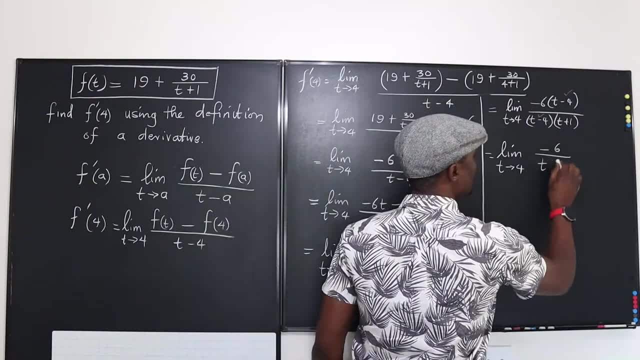 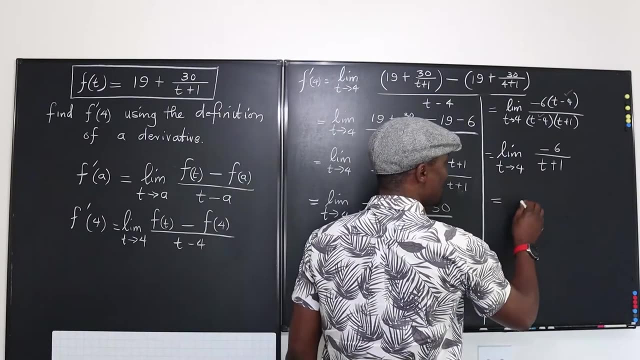 let will be the limit, as t goes to 4, t goes to 4, okay, of negative 6 over t plus 1.. Now we can substitute without worrying about whether we get 0 or not. Well, this is going to be equal to negative.